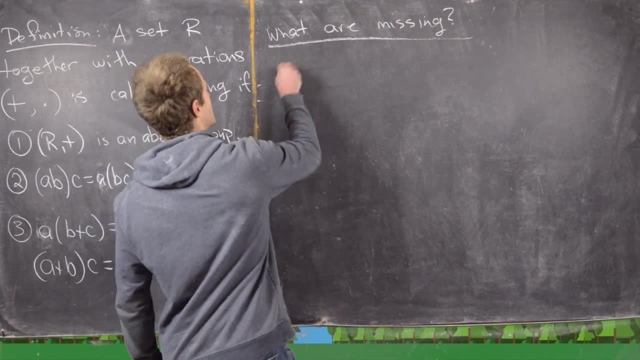 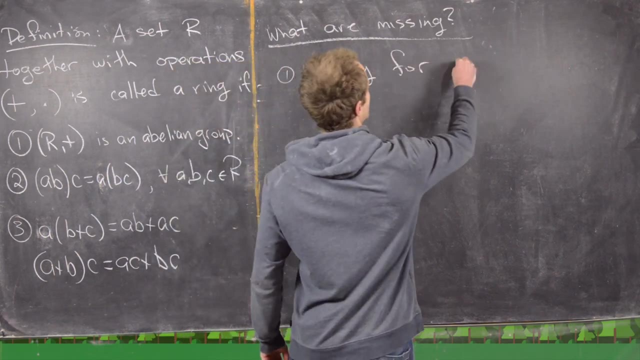 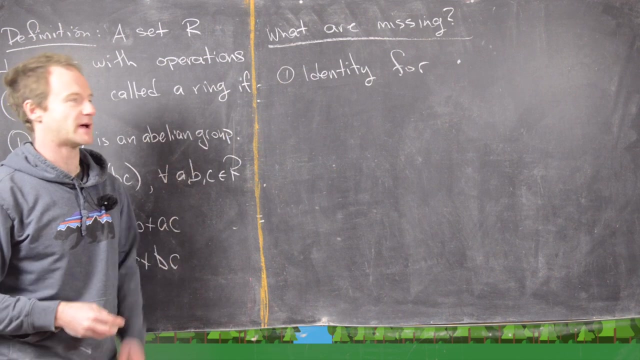 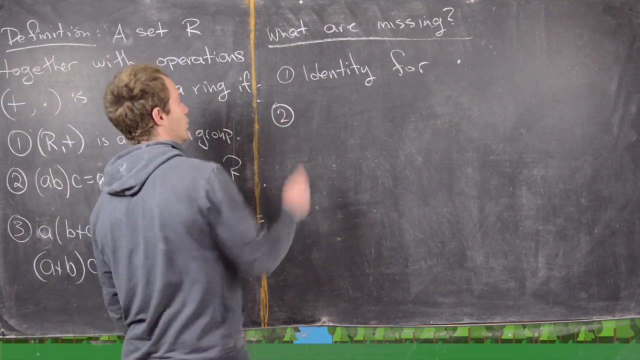 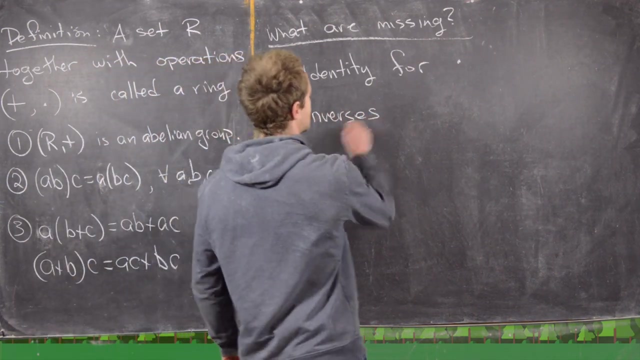 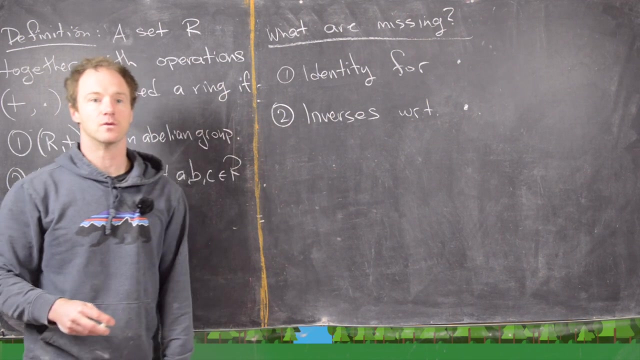 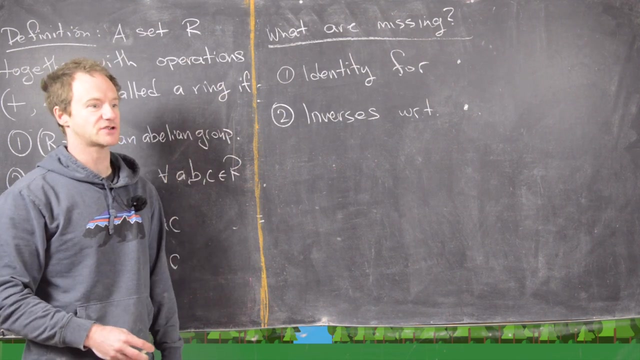 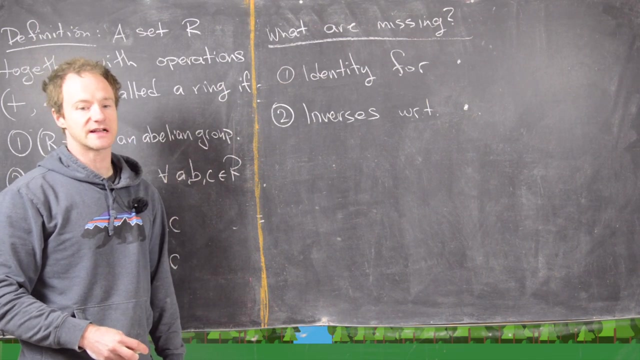 maybe kind of like to have. And that would be the first one would be an identity for the multiplication. And it's true. Sometimes we will have an identity for multiplication. And that'll be a special type of ring. But we don't need that for the structure to be called a ring. And then something that goes along with the identity for multiplication is inverses. And I'll say inverses with respect to this multiplication. So that might be something we also want to have. And what we will see is that we can't have inverses for every element, there's a special element, which will never have an inverse, which we'll see later. But sometimes we will have inverses for everything except for that element. And then maybe one other thing that we would like to have would be 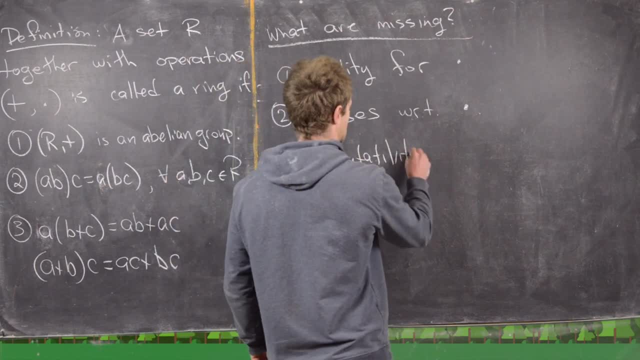 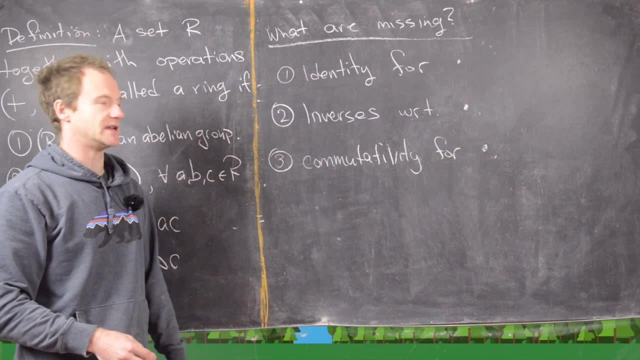 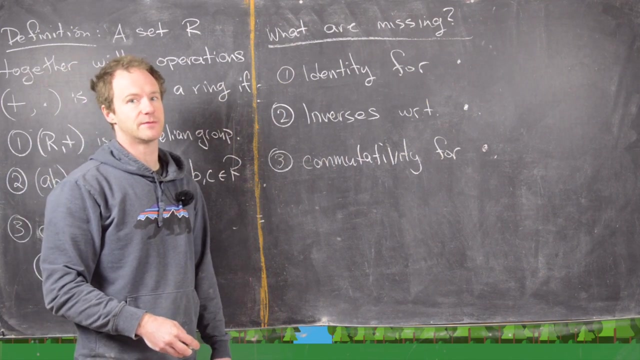 a ring for, for the multiplication operation. So for the multiplication operation. So in o er to be a ring, we do not need commutativity for the or craчикation ampere, we would often have it f nept but we will often have it. Okay, I'll clean up he board and then e will look at some examples. 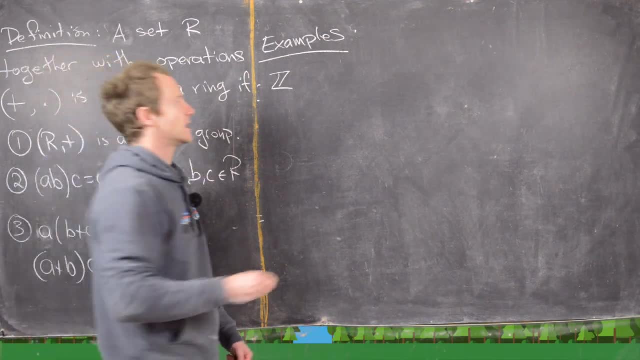 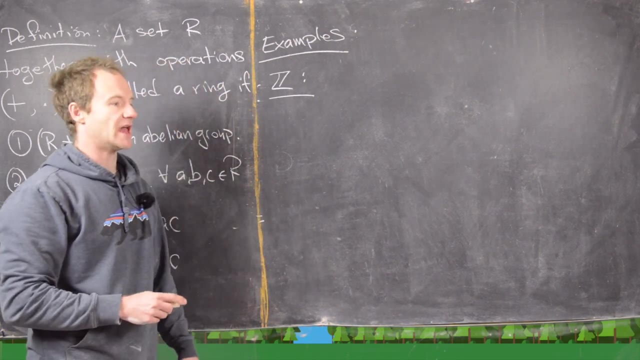 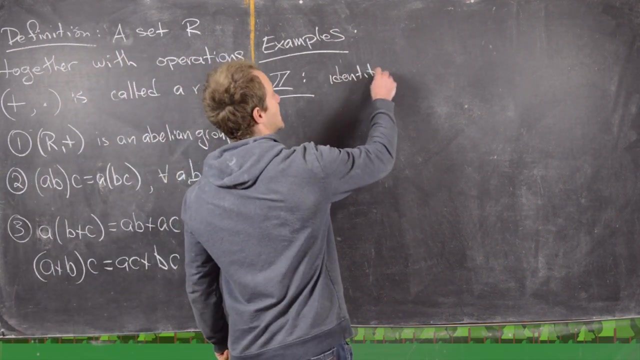 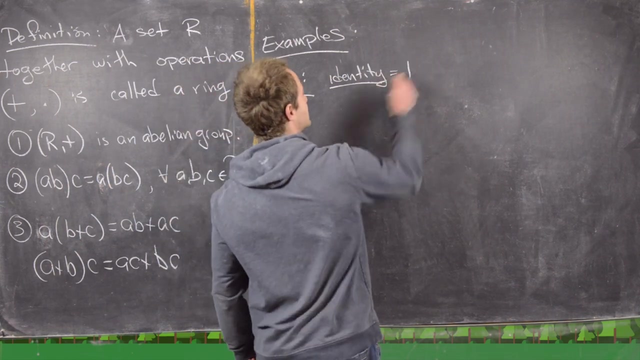 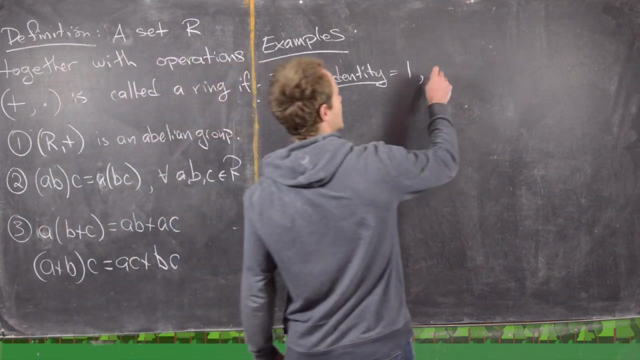 So the first example that I would like to look at is the inte gers and let's notice some things about the inte gers. So I should say what the operations are the opportunities are normal edition and normal d multiplication so now notice here we have an identity and whenever I say identity I mean multiplicative identity because we always have an additive identity which is 0 and the multiplicative identity here is 1 so we in fact do have a multiplicative identity we also have the multiplication 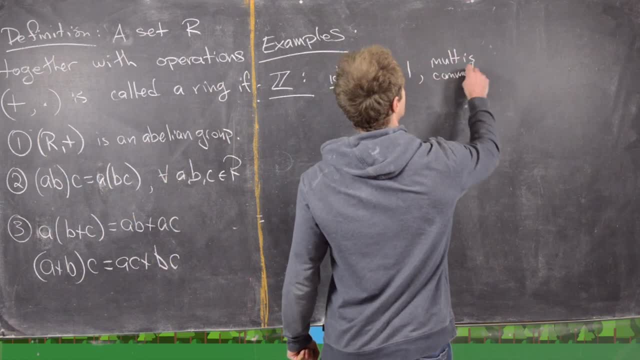 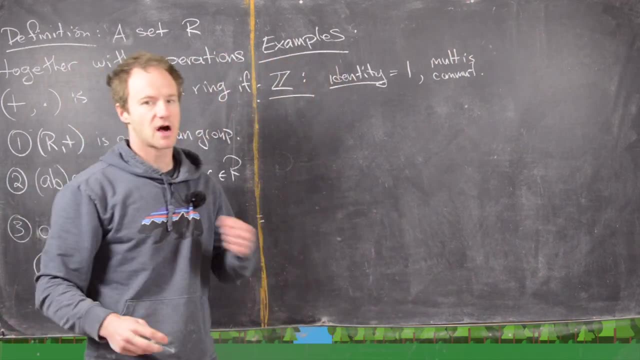 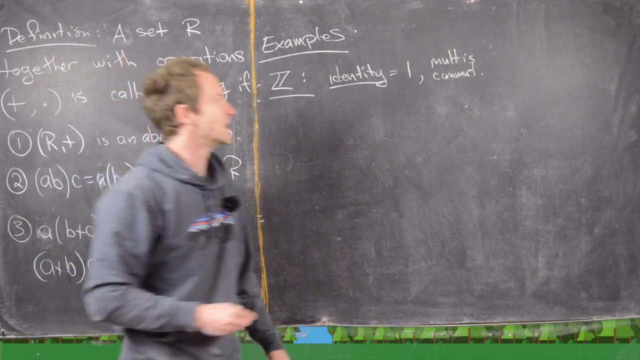 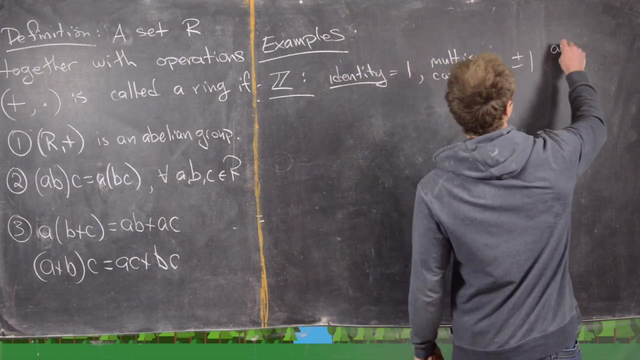 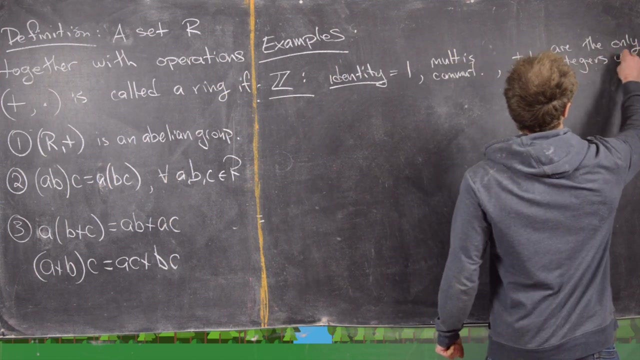 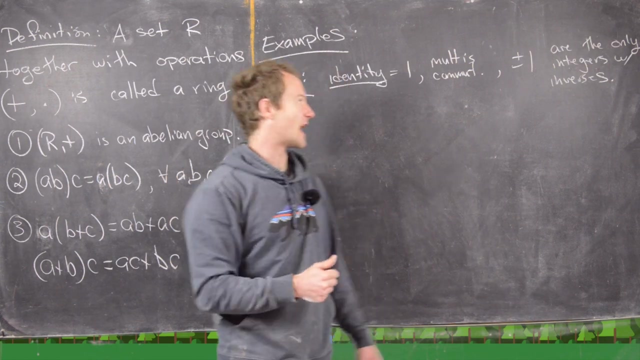 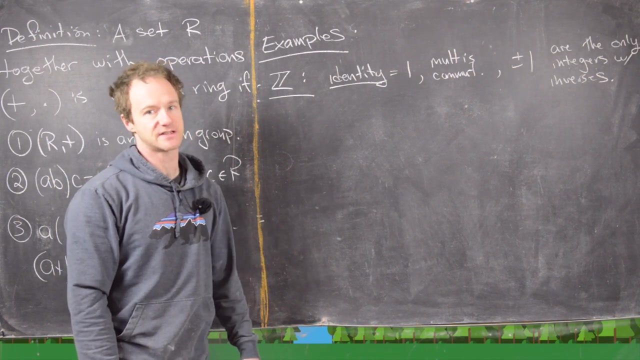 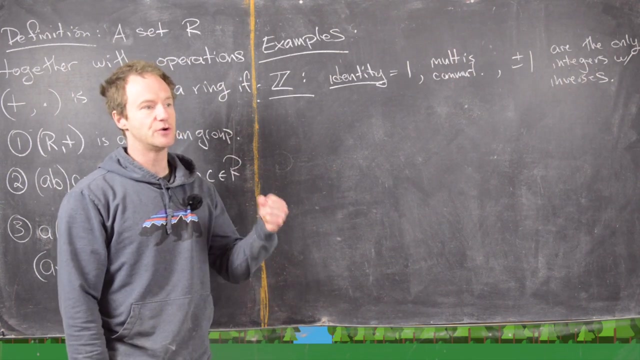 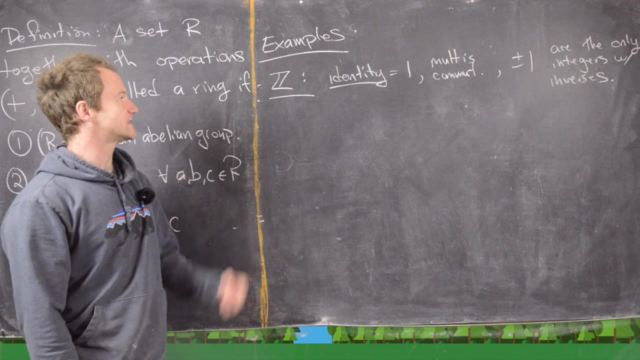 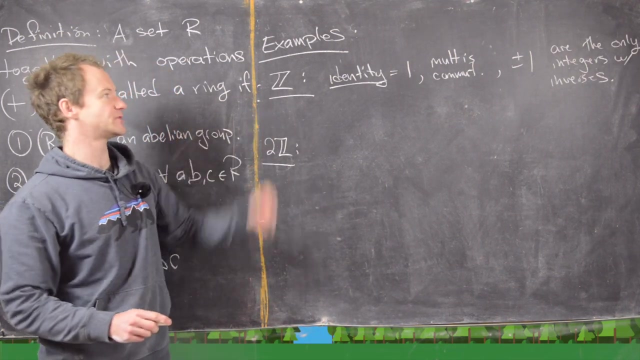 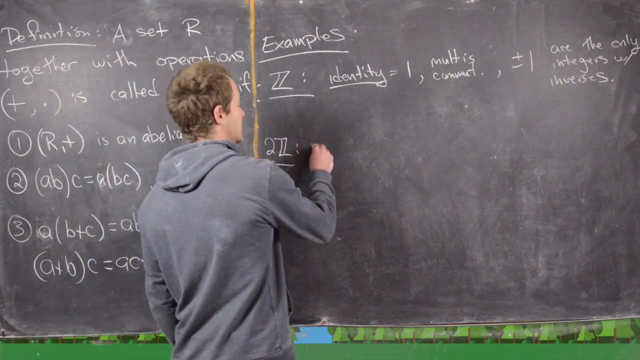 is commutative and generally if it's commutative we call it a commutative ring so the addition is always commutative so whenever we're talking about the commutative of a ring it's always with respect to the multiplication and that's true because we just have numbers here but lots of stuff does not have an inverse in fact plus and minus 1 are the only integers with inverses and what I should say here is again that's with respect to multiplicative because everything's going to have an additive and inverse so notice 1 is its own inverse that's true because it's the identity and negative 1 is its own inverse and that's because negative 1 times negative 1 is positive 1 but everything else doesn't have an inverse notice the inverse of 2 is 1 half but that's outside of the integers okay good so now let's go from there and let's say maybe 2z so that's going to be a substructure of Z and notice that we get some of these but not all of these so notice there's going to be no identity in this case that's because we took away 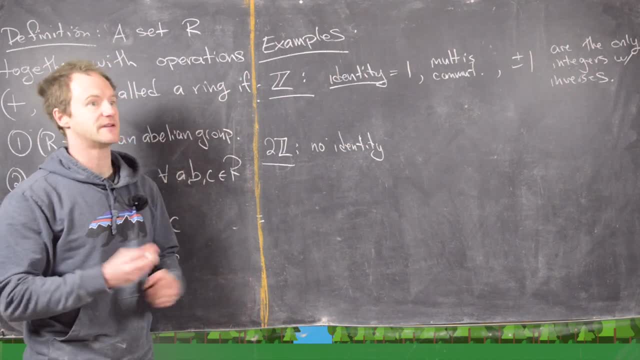 the number 1 notice here everything is even we just have 0 plus minus 2 plus minus 4 plus minus 6 and so on and so forth 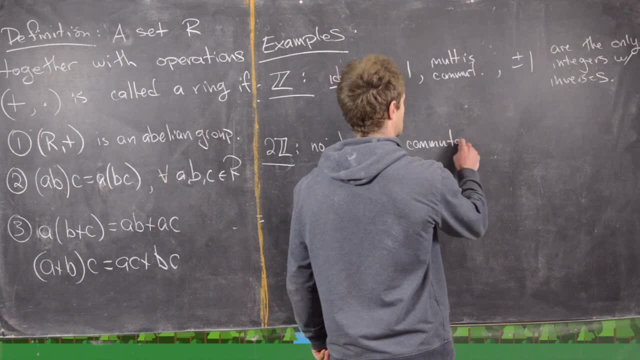 we do have commutativity so it is commutative but then nothing 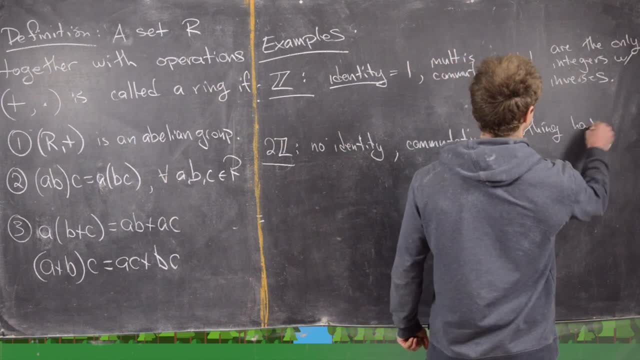 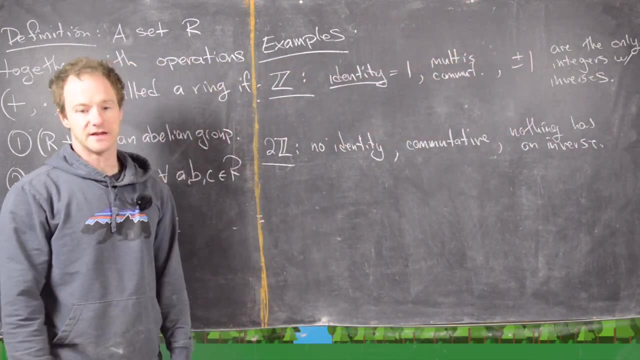 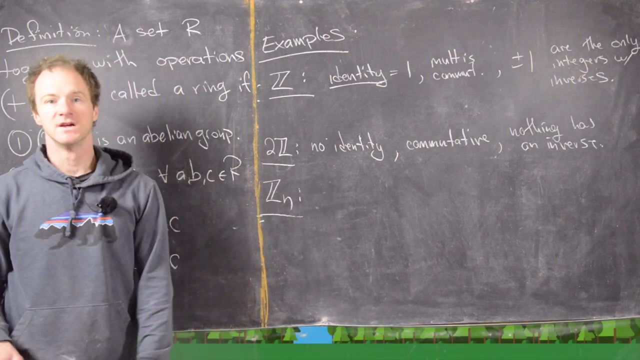 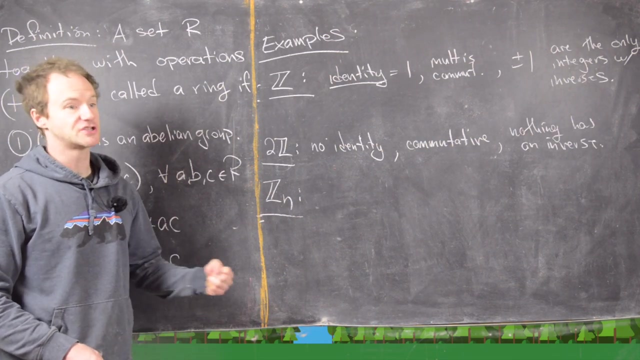 has an inverse so that's our setup for 2z okay so now let's look at another thing let's maybe look at Zn okay so in other words we have the integers modulo n we have multiplication modulo n and addition modulo n so we do have an identity in this case 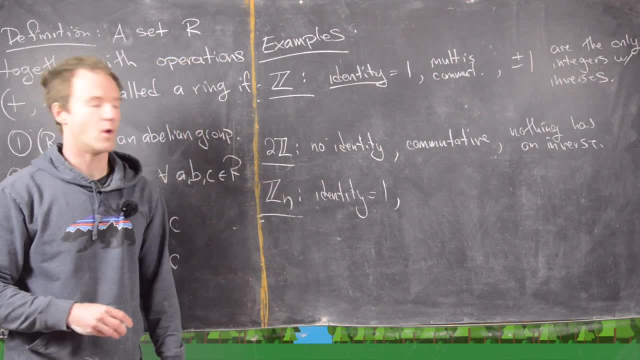 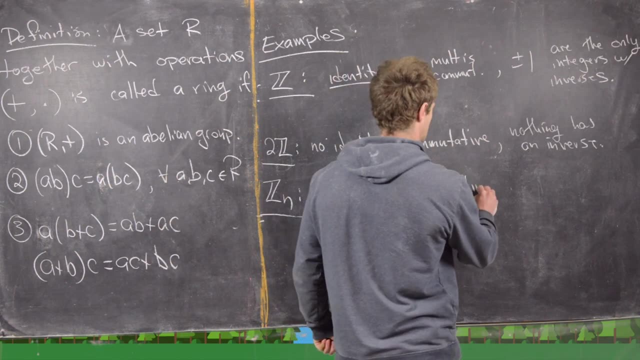 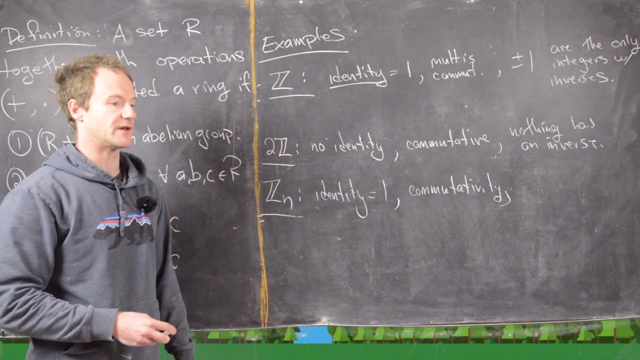 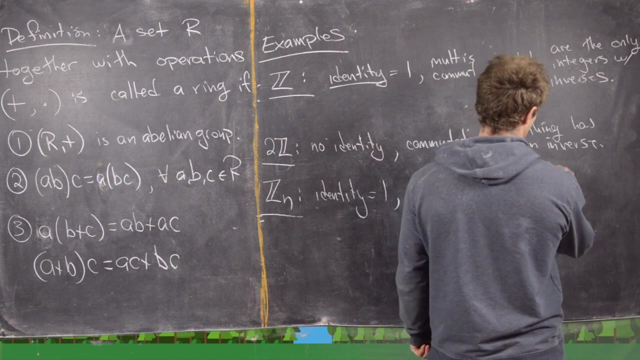 and that is the equivalence class of 1 mod n we do have commutativity and then some stuff has inverses and from what we know about group theory everything that's relatively prime has an inverse so we'll say that M inverse in Zn exists if and only if 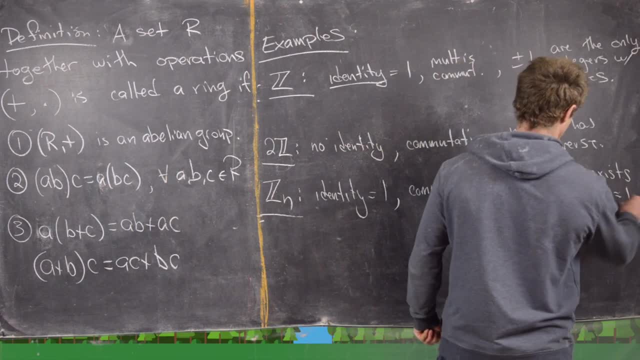 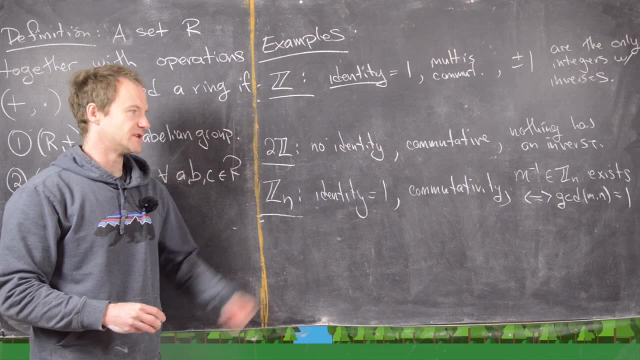 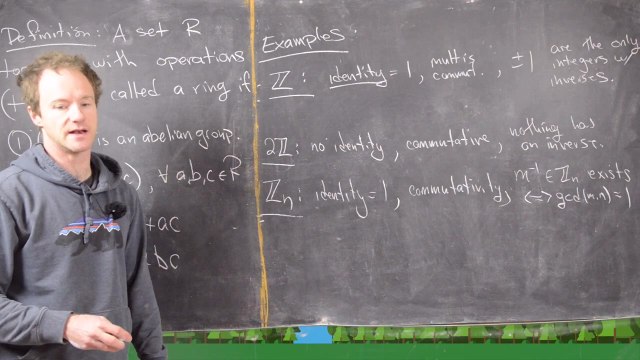 the GCD of M and n equals 1 in other words M is in un the group of units modulo n so we'll look at this ring a lot more carefully later but just as a brief overview that's what we get for Zn 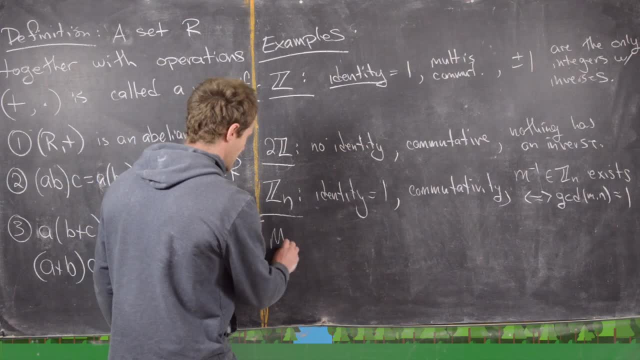 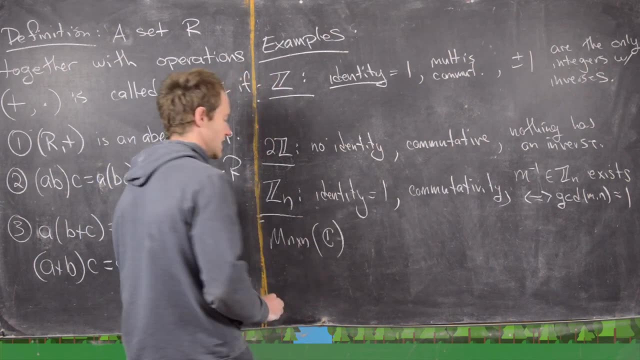 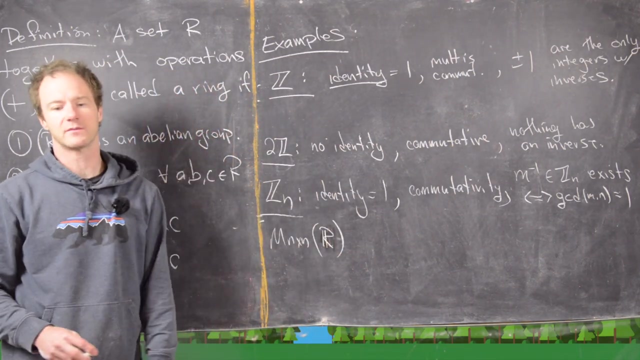 ok so let's look at another one maybe M n by n and then maybe we could go over any ring but what I want to do is maybe just over the complex numbers or the real numbers if you're more familiar with the real numbers or the rational numbers and then we have matrix addition and matrix multiplication 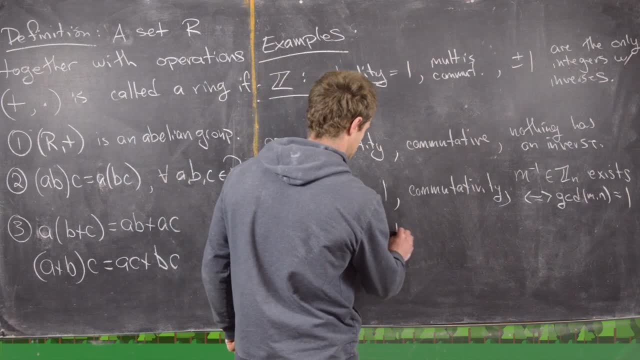 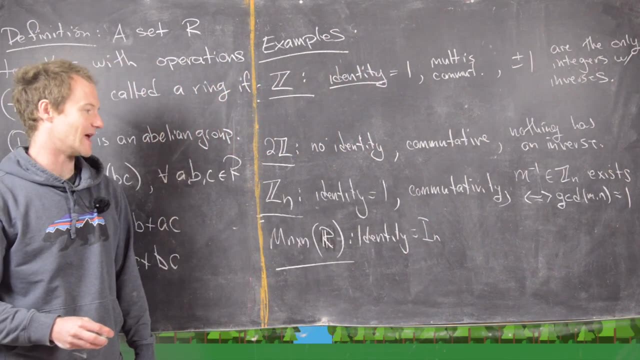 ok so we have an identity here and that identity is going to be the N by n identity matrix so I'll just call that thing In and then not commutative ..... ...... ...... 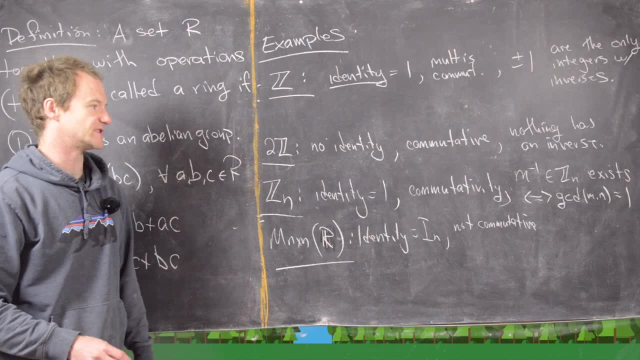 So it's well known from linear algebra that matrix multiplication does not commute. But then a bunch of things do have multiplicative inverses. And let's say it like this. 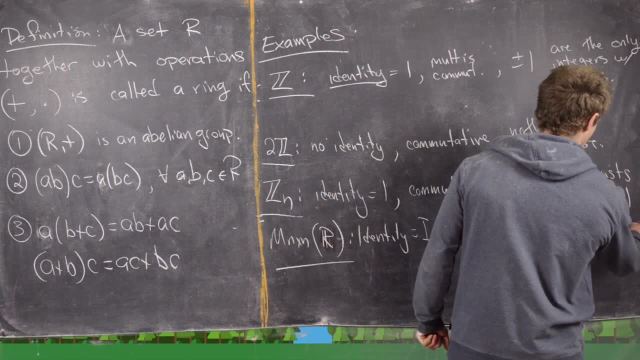 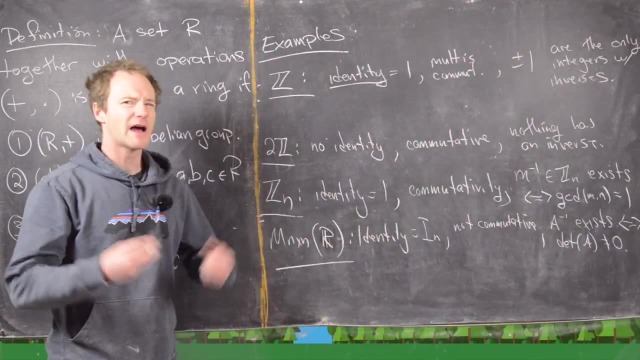 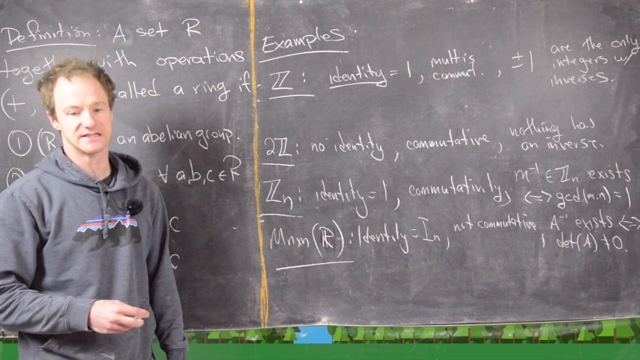 So A inverse exists if and only if the determinant of A is not equal to 0. And then by the invertible matrix theorem, which is something you learn in linear algebra, there are lots of ways to say if A inverse exists or not. 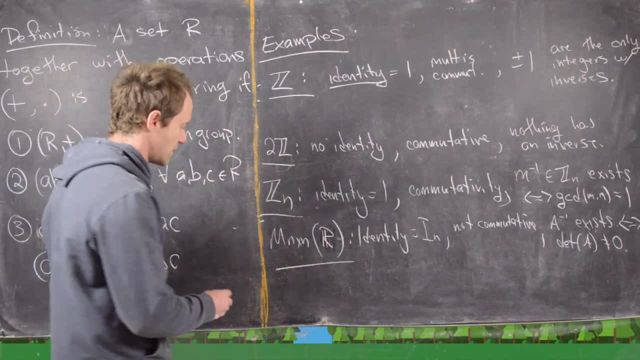 Okay, so I want to look at one more before the end of this video. And that would maybe be Z join X.